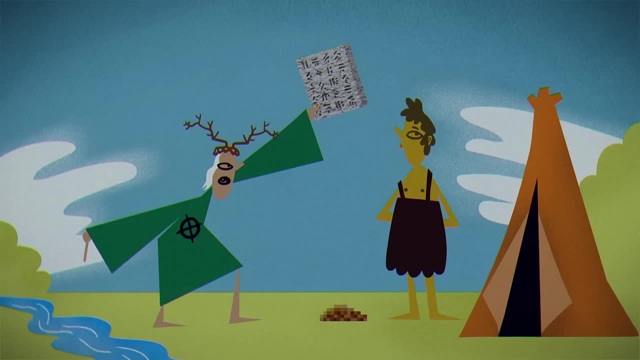 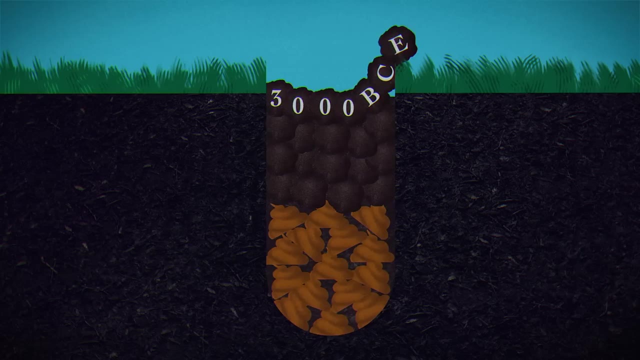 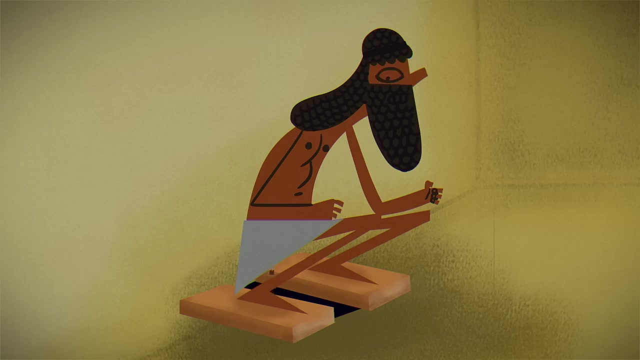 contain instructions for keeping waste away from drinking water and campsites. waste management took a more familiar shape as early as 3000.. Ancient Mesopotamian settlements often had clay structures made for squatting or sitting in the most private room of the house. These were connected to pipes which used running water. 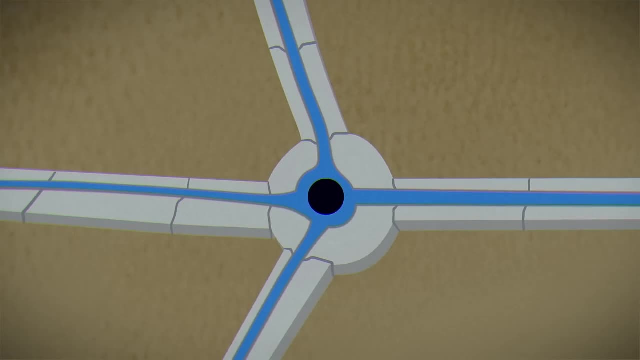 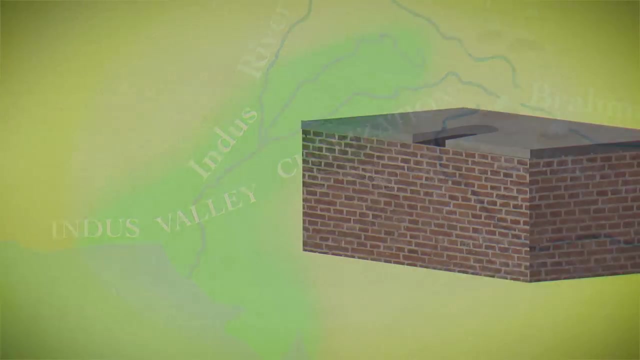 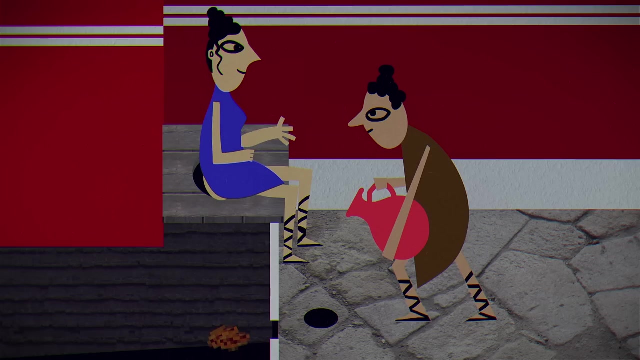 to move waste into street canals and cesspits. Water infrastructure like this flourished in the Bronze Age and in some parts of the Indus Valley nearly every house had a toilet connected to a city-wide sewage system. Ancient Cretan palaces even offered a manual flushing option. 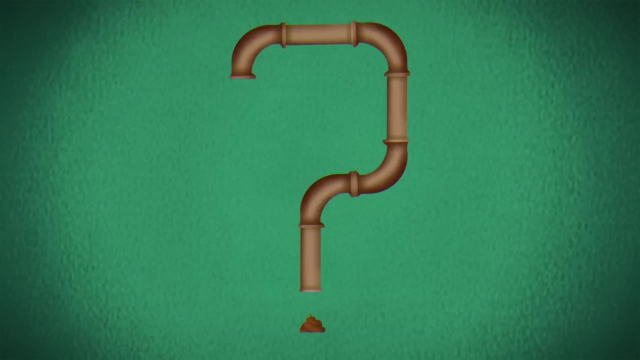 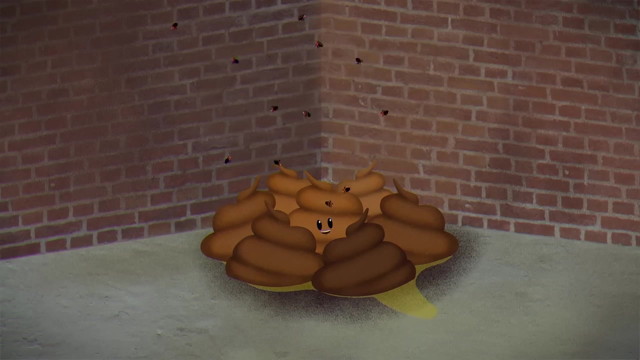 Researchers can't say for certain what inspired these early sewage systems, but we do know that waste management is essential for public health. Untreated sewage is a breeding ground for dangerous microorganisms, including those that cause cholera, dysentery and typhoid. 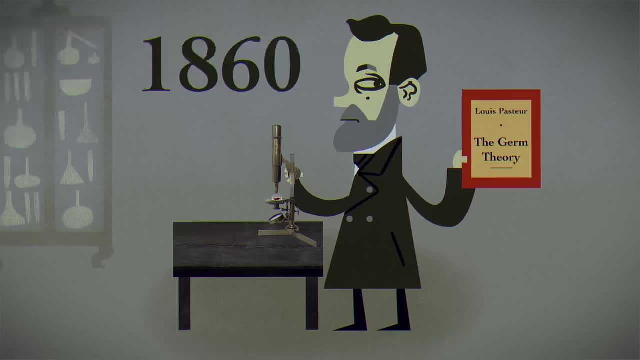 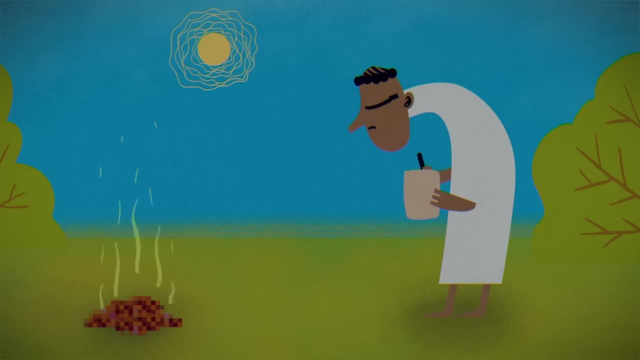 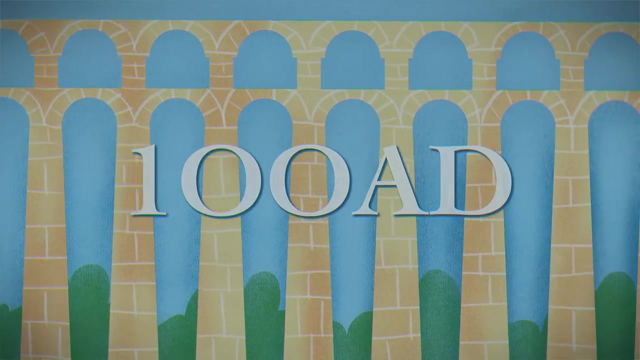 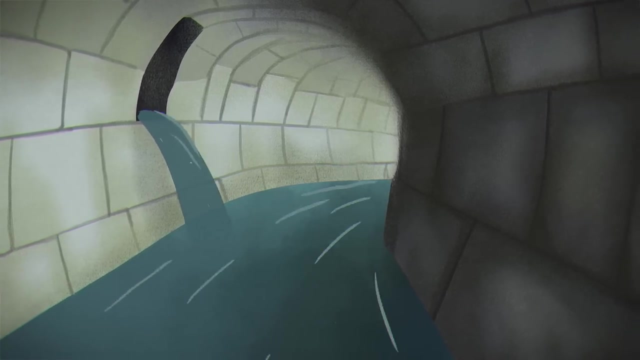 It would be several millennia before scientists fully understood the relationship between sewage and sickness, but the noxious odors of sewage have recorded associations with disease as early as 100 BCE And by 100 AD. more complex sanitation solutions were emerging. The Roman Empire had continuously flowing aqueducts dedicated to carrying waste outside. 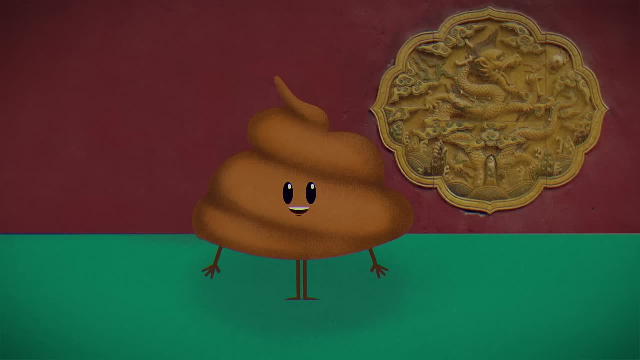 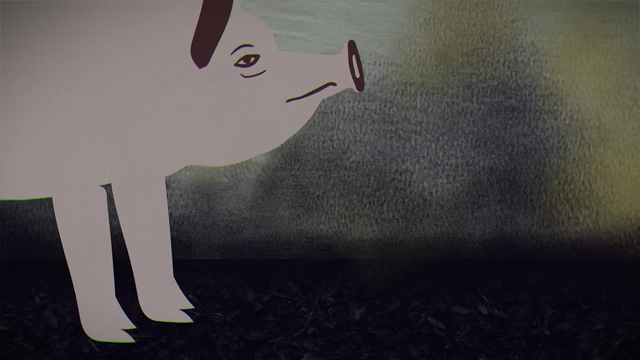 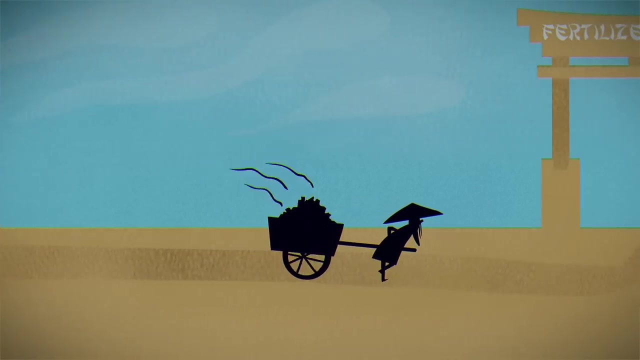 city walls. Chinese dynasties of the same period also had private and public toilets. except their, waste was immediately recycled. Most household toilets fed into pigsties, and specialized excrement collectors gathered waste from public latrines to sell as fertilizer. 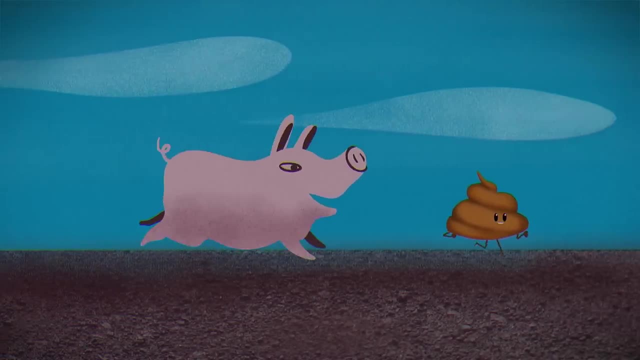 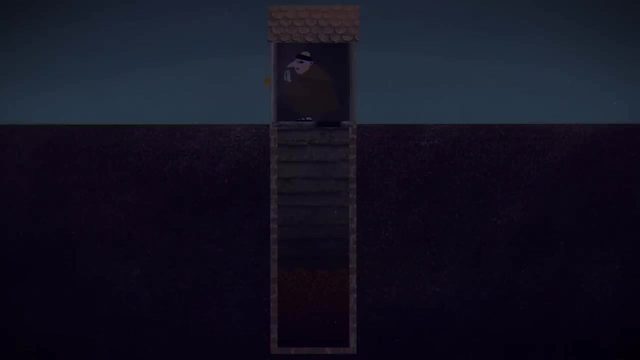 In China, this tradition of waste management continued for centuries, but in Europe the fall of the Roman Empire brought public sanitation into the Dark Ages. Pit latrines called gongs became commonplace and chamber pots were frequently dumped into the street. 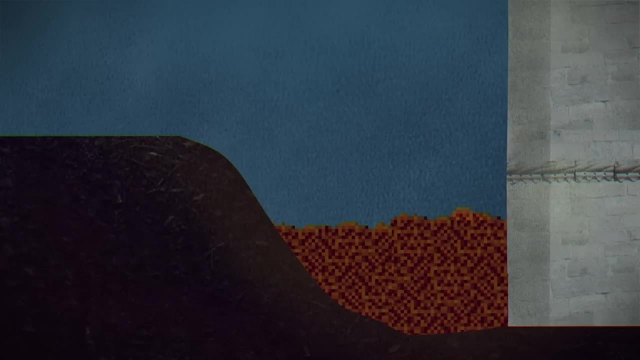 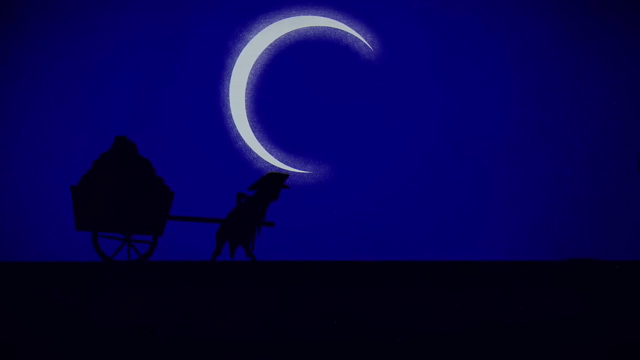 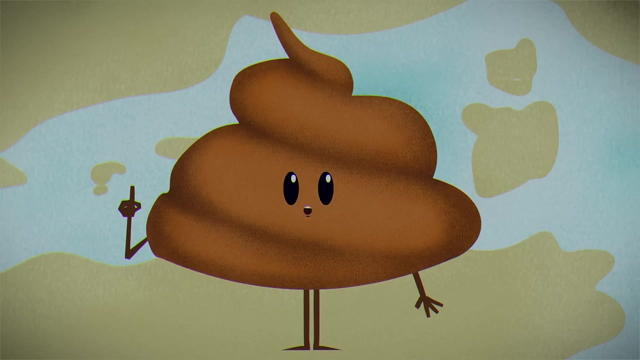 Castles ejected waste from tall windows into communal cesspits At night. so-called gong farmers would load up the waste before traveling beyond city limits to dump their cargo. Europe's unsanitary approach persisted for centuries, but toilets themselves underwent some major changes By the late Middle Ages most wealthy. 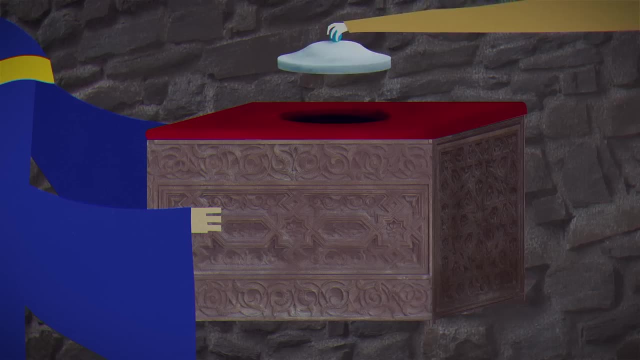 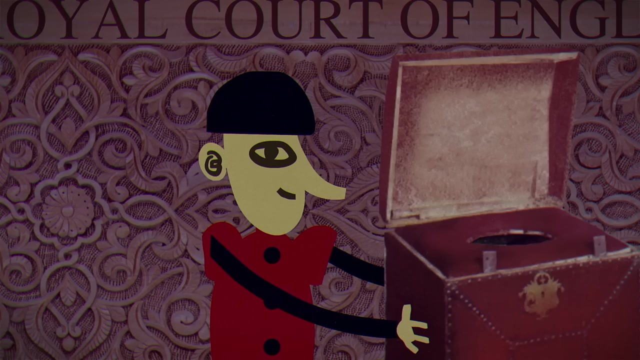 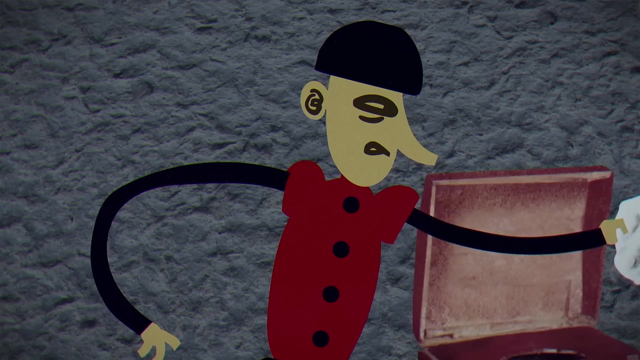 families had commode stools, wooden boxes with seats and lids, And in the royal court of England, the commodes were controlled by the groom of the stool. In addition to monitoring the king's intestinal health, the groom's intimate relationship with the monarch made him a surprisingly influential. 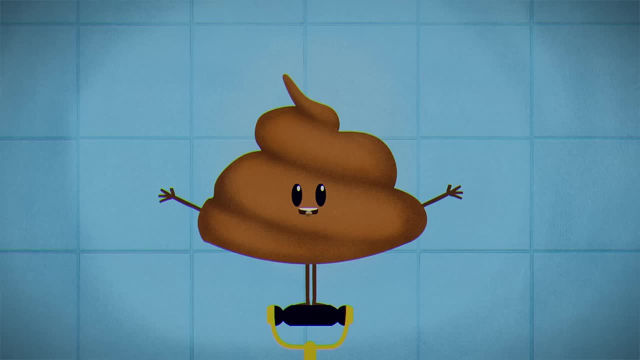 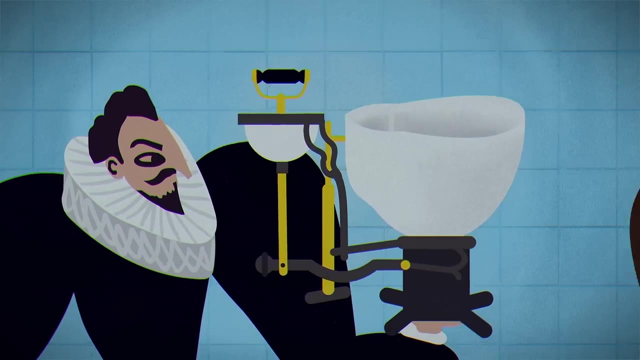 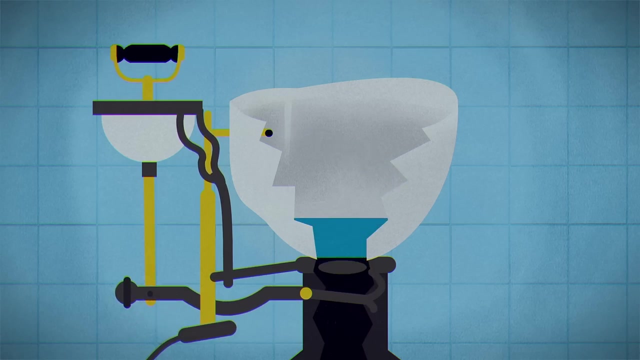 figure. The next major leap in toilet technology came in 1596, when Sir John Harrington designed the first modern flush toilet for Queen Elizabeth. Its use of levers to release water and a valve to drain the bowl still inform modern designs, but Harrington's invention stank of sewage. 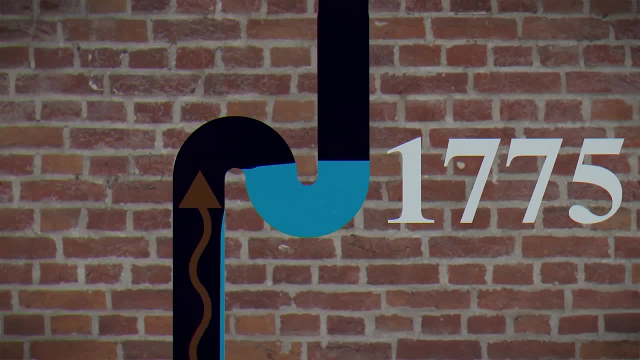 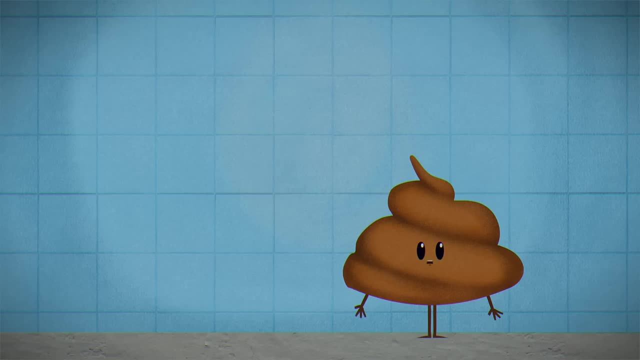 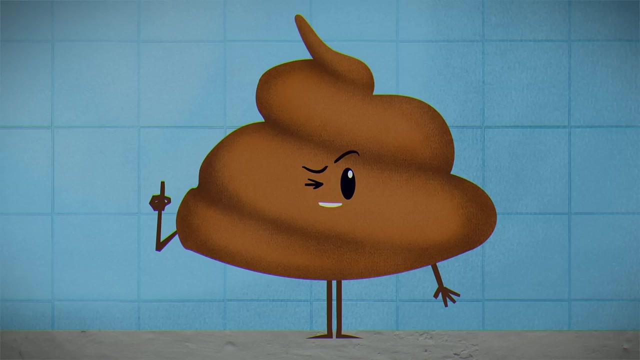 Thankfully, in 1775, Scottish inventor Alexander Cumming added a bend in the drain pipe to retain water and limit odors. This so-called S-trap was later improved into the modern U-bend by Thomas Crapper, though the term crap predates the inventor by several centuries, By the turn of the 19th. 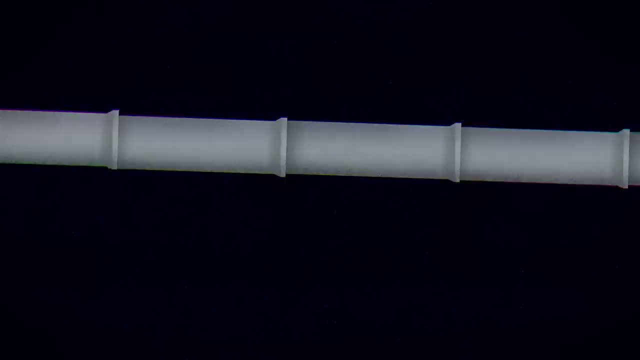 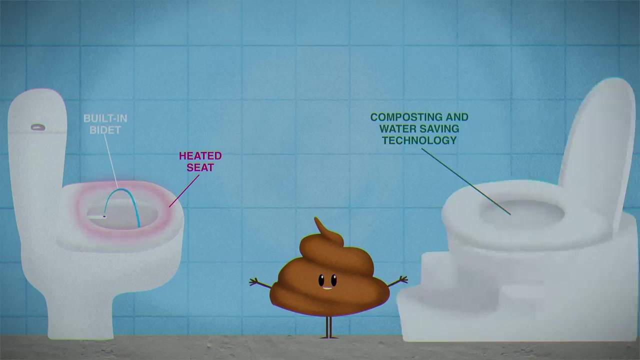 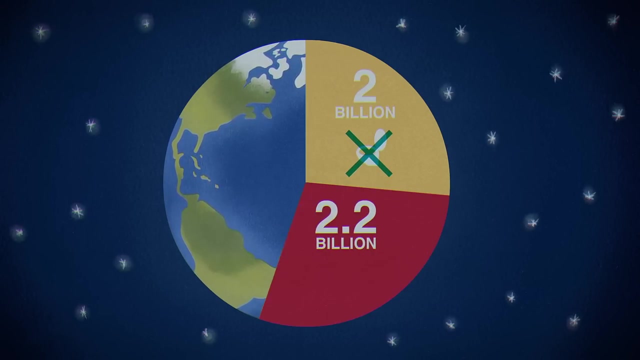 century, many cities had developed modern sewage infrastructure and wastewater treatment plants, and today toilets have a wide range of features, from the luxurious to the sustainable. But roughly 2 billion people still don't have their own toilets at home and another 2.2 billion don't have facilities that properly manage their waste. 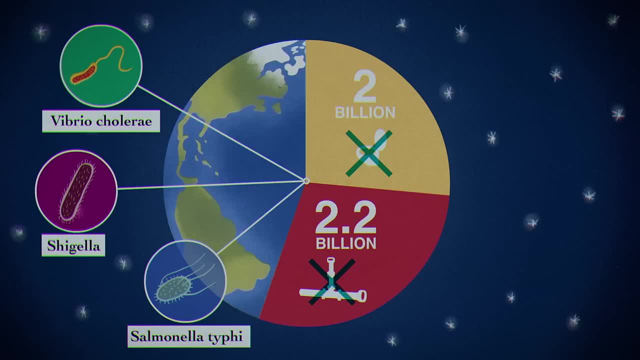 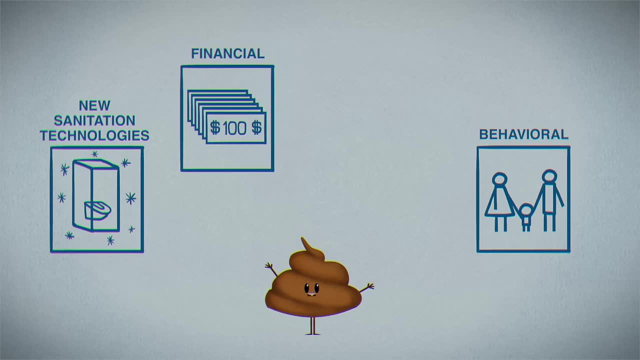 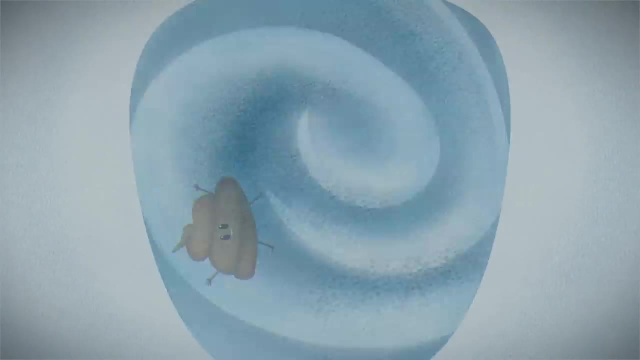 putting these communities at risk of numerous diseases. To solve this problem, we'll need to use new technologies and address the behavioural, financial and political issues that produce inequity throughout the sanitation pipeline, So with all the humans and animals in the world. 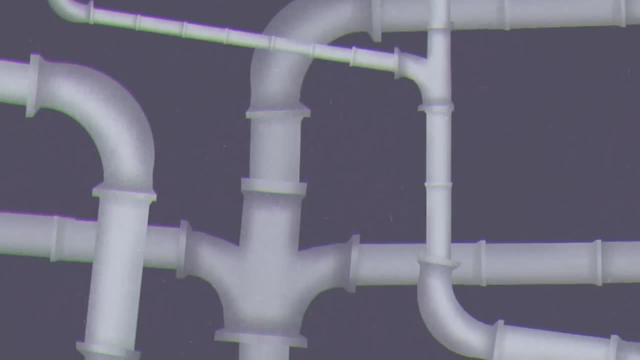 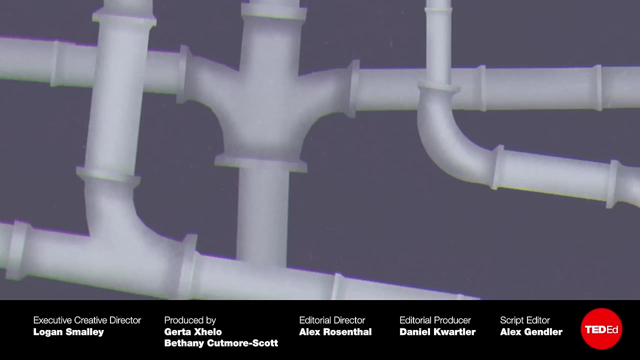 defecating daily. why isn't the planet covered in an endless stream of faeces? Check out this video on the humble dung beetle, who you can thank for their mighty clean-up skills.